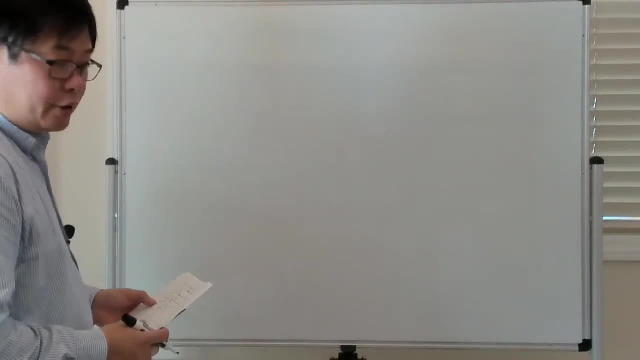 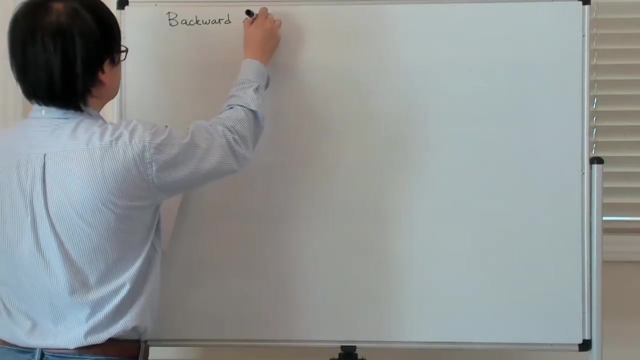 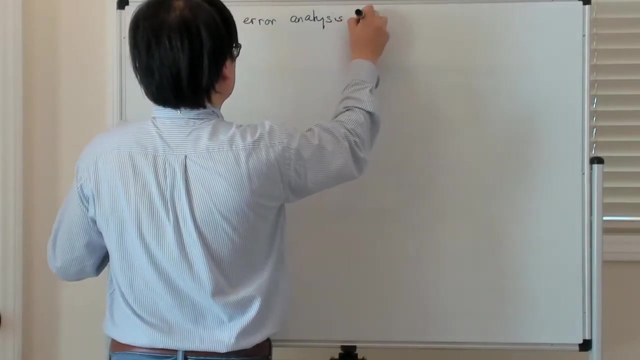 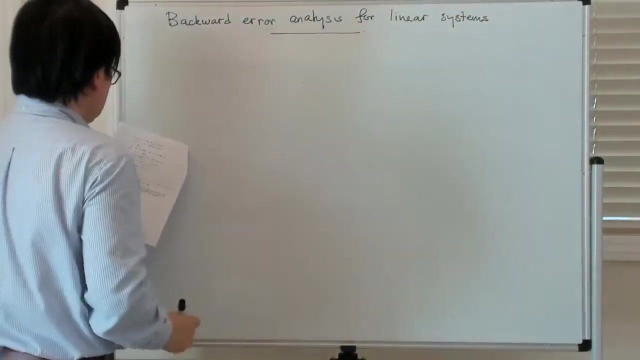 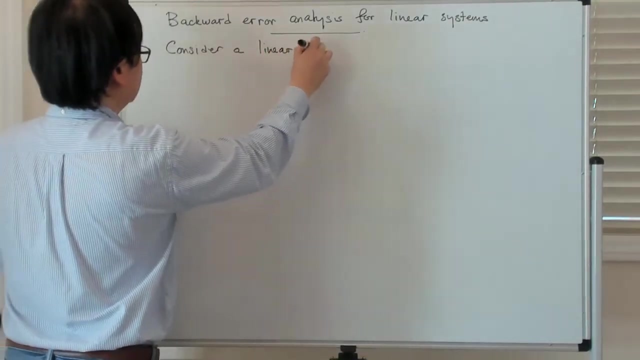 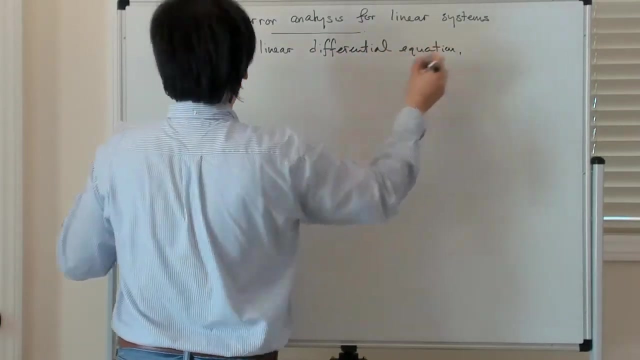 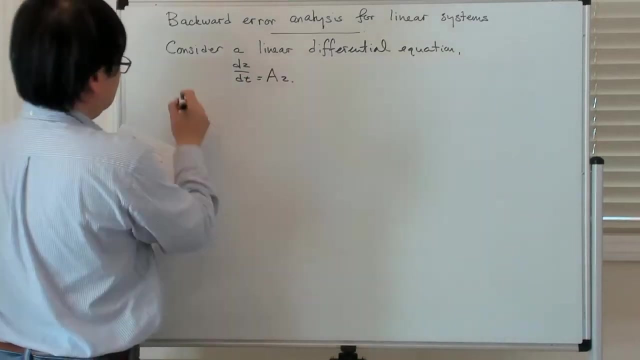 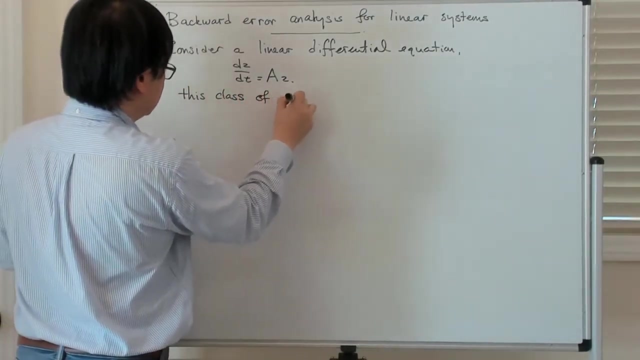 like to illustrate what goes into the process of backward error analysis. Okay so, this is backward error analysis for linear systems. Okay, so, let's consider a linear differential equation. Okay, so, dz, dt is az, And the reason, as I said, is that this class of problems allow us to satisfy. 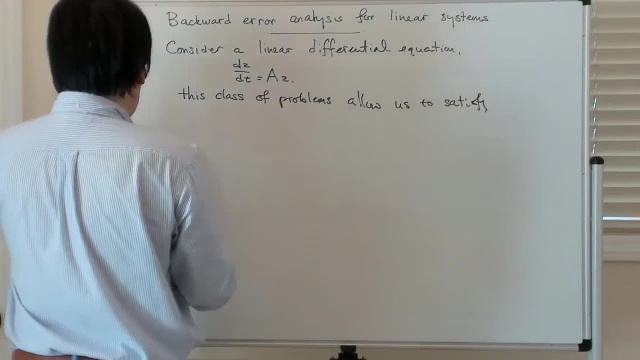 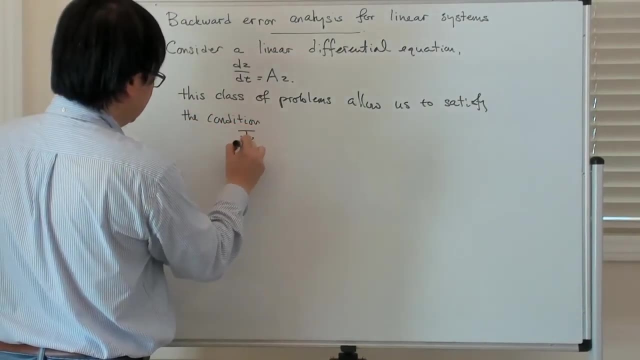 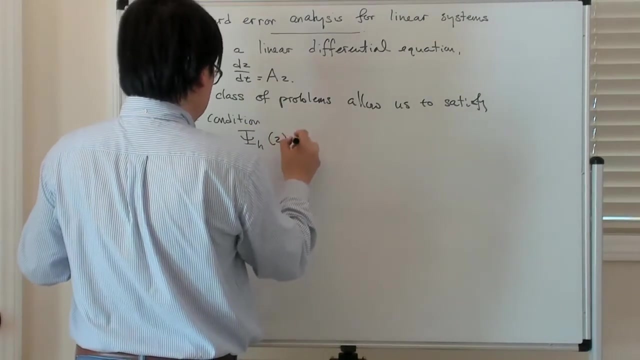 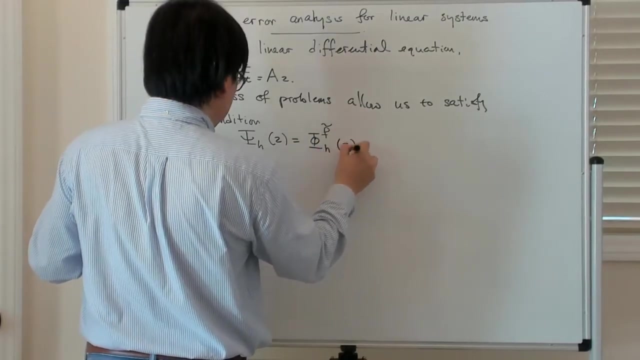 the differential equation. Okay, so dz, dt is the condition that the one-step method applied to this sort of differential equation is equal to the exact time H-flow of a modified vector field. Okay, so what that means is that you can actually compute these. 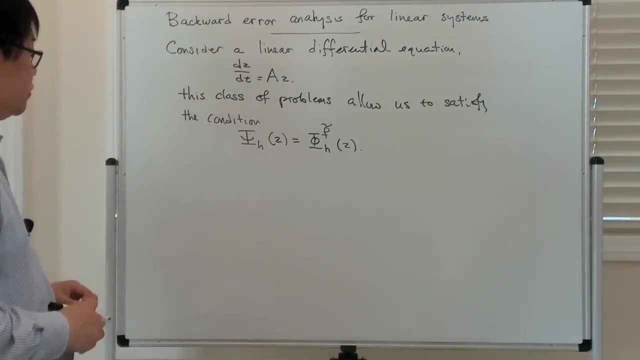 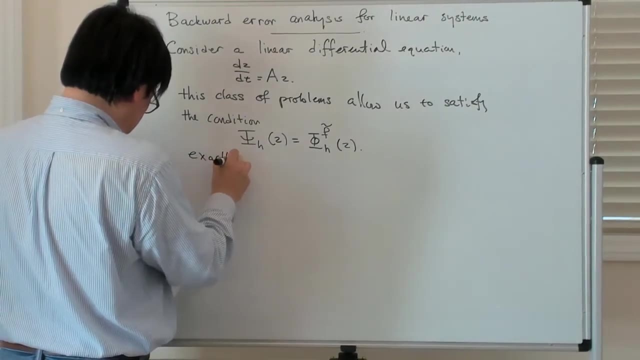 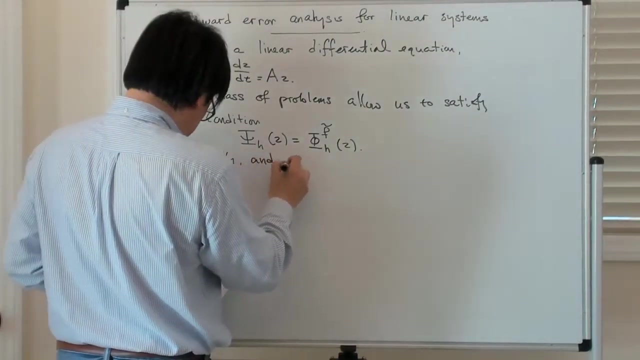 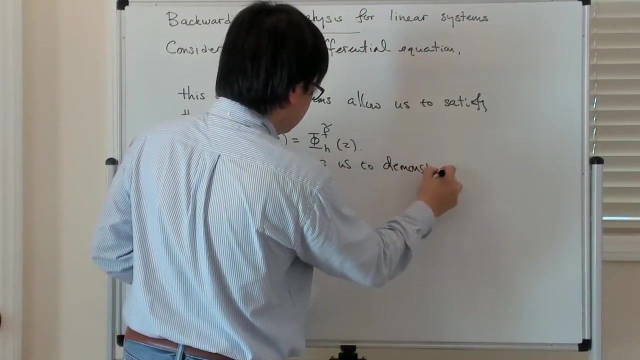 terms by terms. It's like the terms give you a series which can give you a series, you a series which converge, it's like, and everything sort of gives you something which is well-defined okay. so this class allows you to satisfy this condition exactly and allows us to demonstrate the basic ideas. 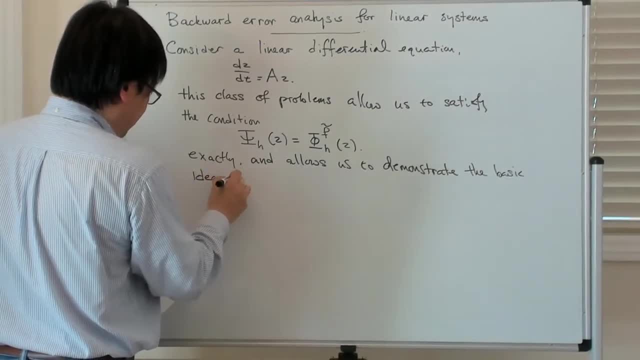 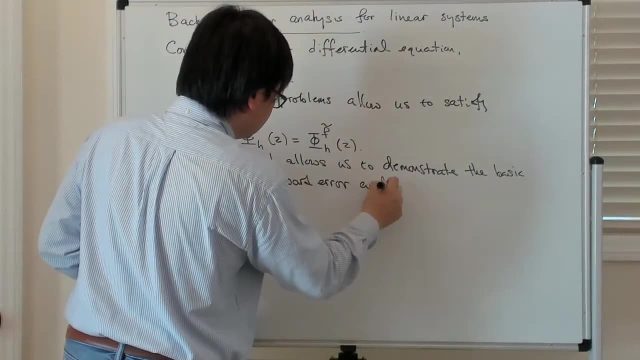 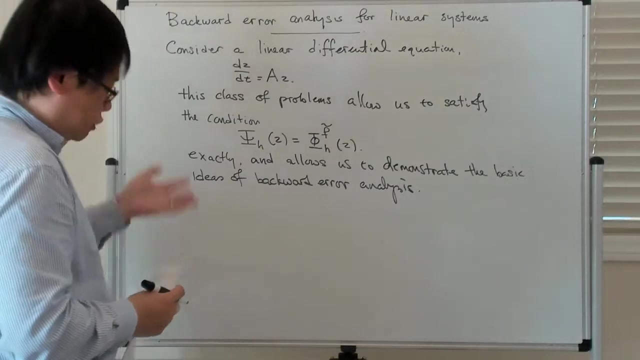 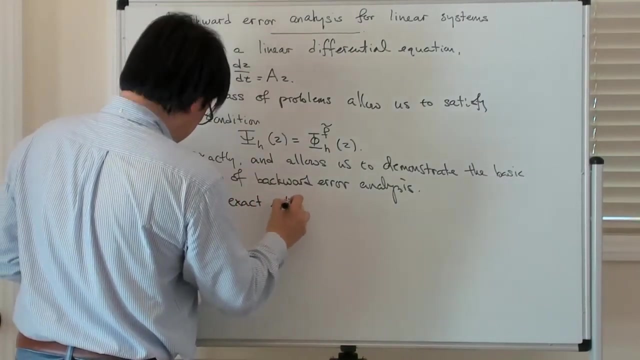 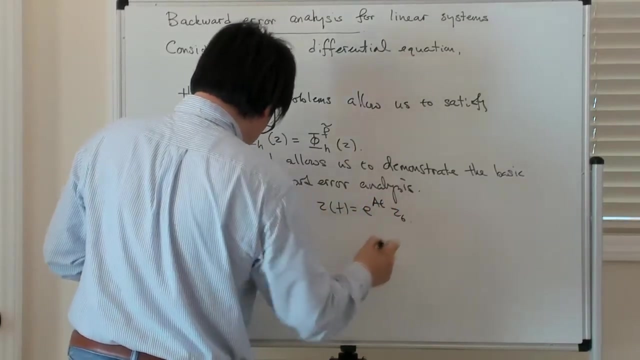 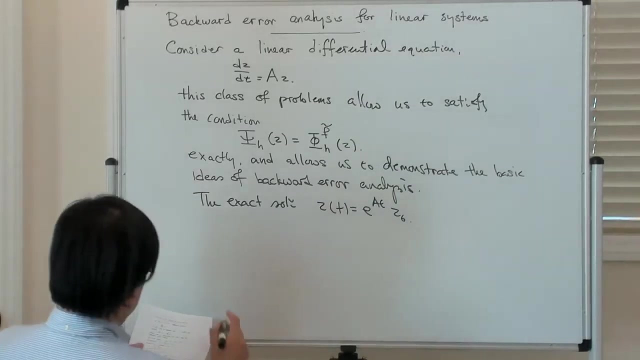 of backward error analysis. okay, all right. so of course you know that if you have a linear differential equation, you know what the exact answer is, right. so the exact solution, of course, is nothing more than Z of T. is e to the E, a t, z, 0. and then your discretization. right, a discretization, let's say Z, n. 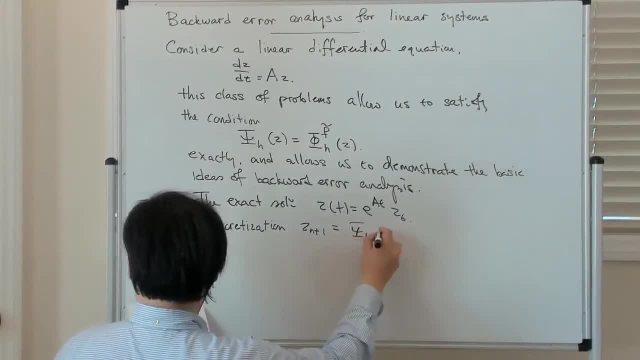 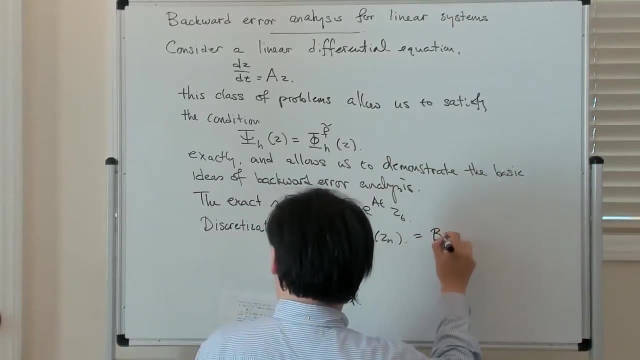 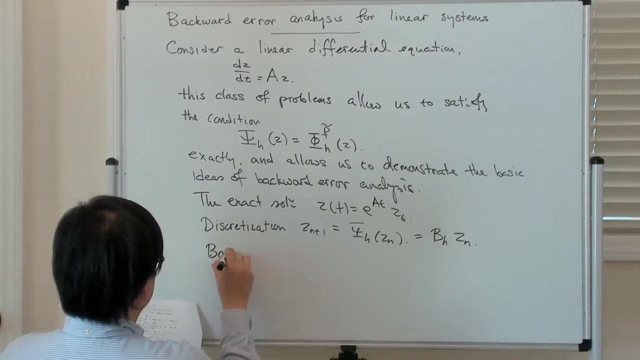 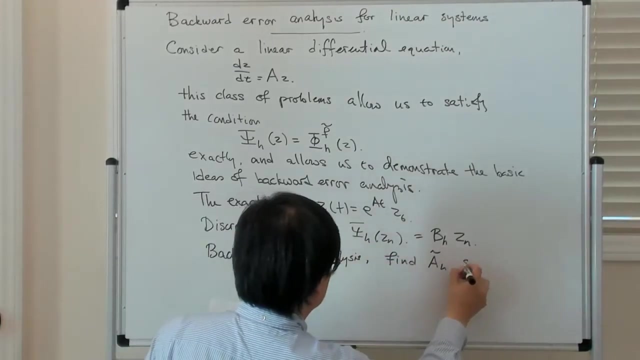 plus 1 is equal to this numerical one step method. apply to see n, which is in general some matrix, let's say B, which depends on H. applied to CNN, you, you And then. so backward error analysis requires you to find a h tilde such that right c, n is equal to e to the t n. 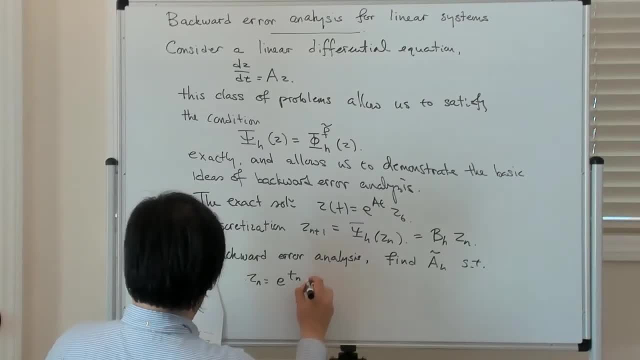 So a h tilde applied to z 0, right, and in particular right where t n is of course just n times h, and then, in particular, for n equals 1, right. we have that the one step method applied to z 0 is of course just b h, z 0,, which is of course a h tilde. 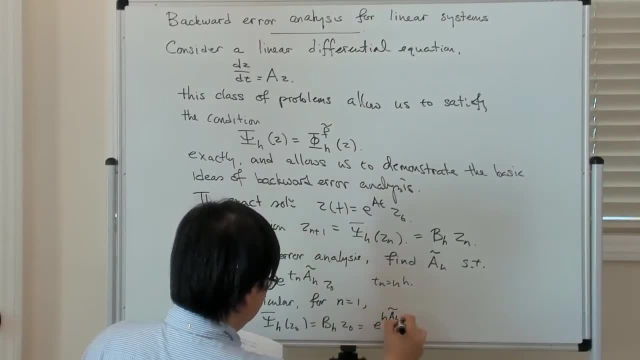 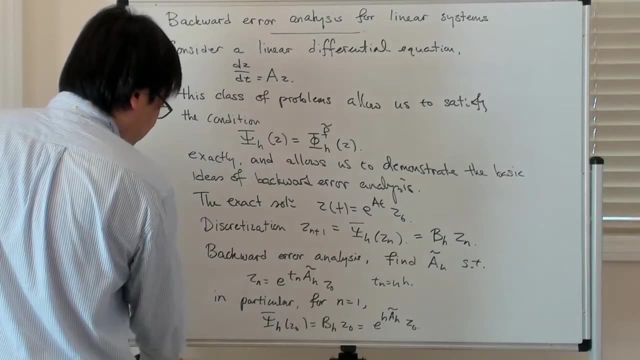 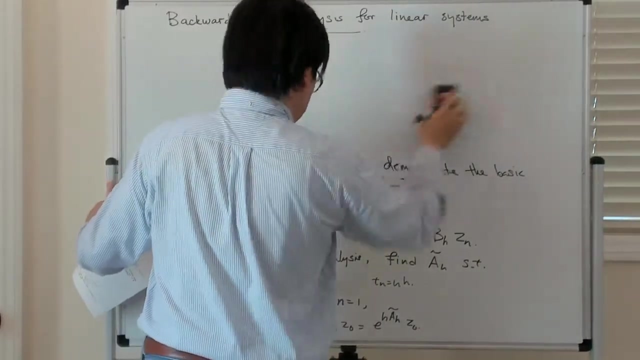 So a h tilde has to be e to the h a tilde, h applied to z 0.. So that allows you to solve for what a h tilde has to be right. Maybe not too exciting, but yeah, it's easy to show what it has to be. 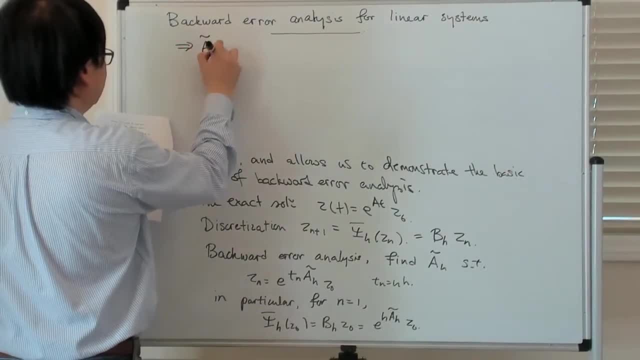 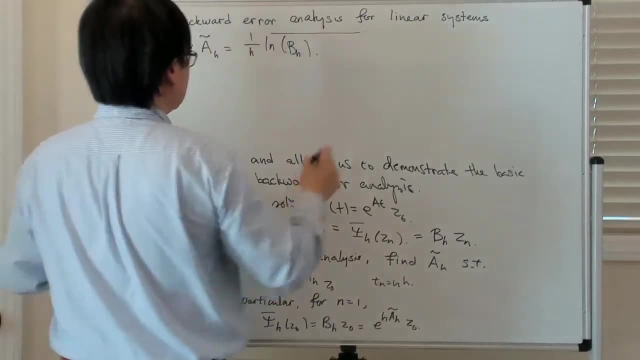 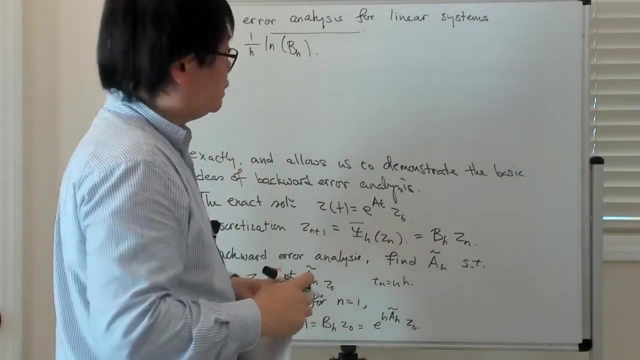 So this implies that a h tilde is equal to just 1 over h, the natural log of b h right. And, of course, the same way that you defined the matrix exponential in terms of looking at the series expansion for the exponential, you do the same thing for the natural log of a matrix right. 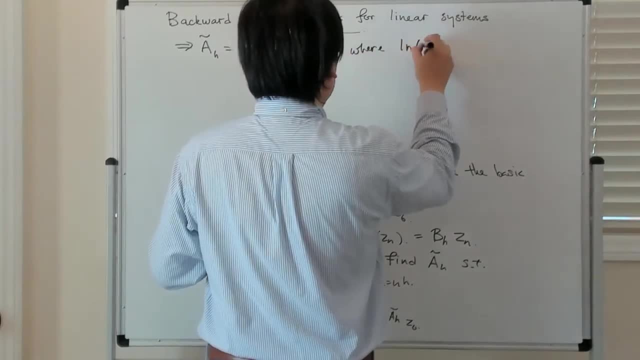 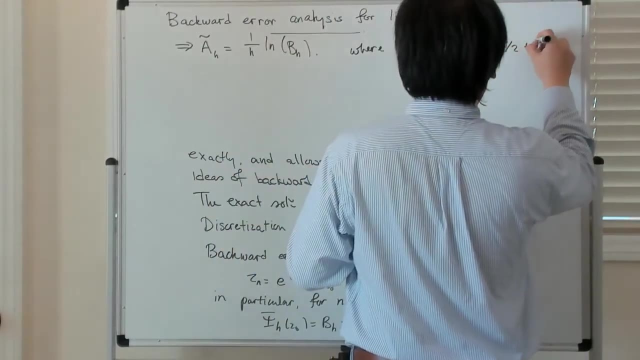 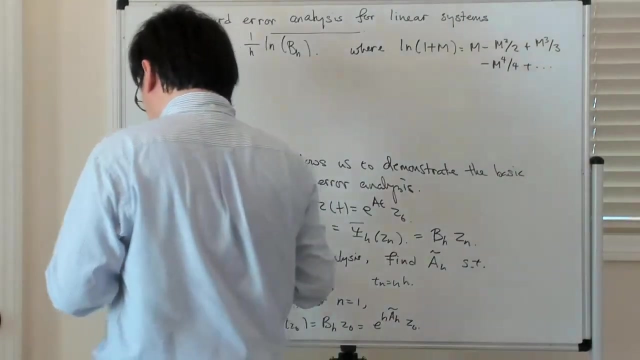 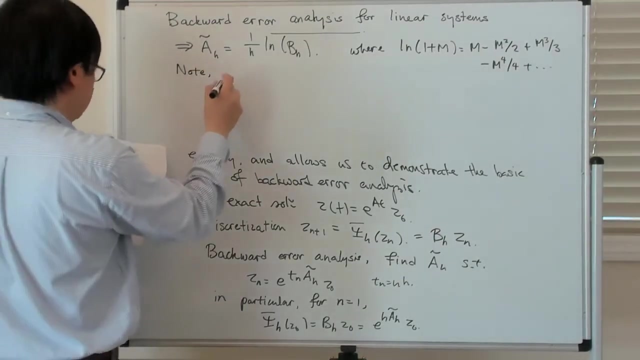 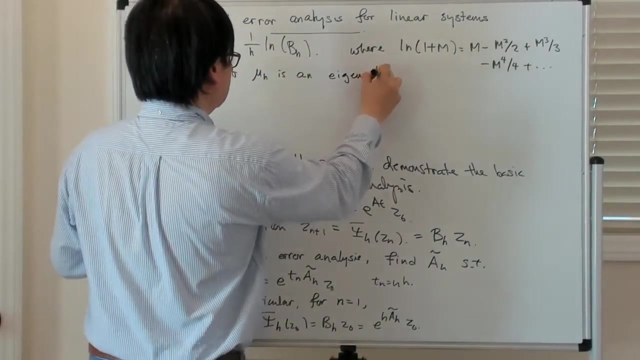 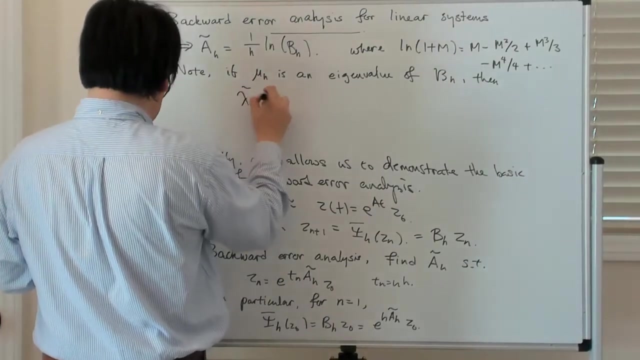 So where natural log of 1 plus m goes to m minus m, squared over 2 plus m, cubed over 3 minus m, to the 4 over 4. And so on. So note the following: right, if mu h is an eigenvalue of b h, then right lambda h tilde, which is 1 over h, natural log of mu h, right is an eigenvalue. 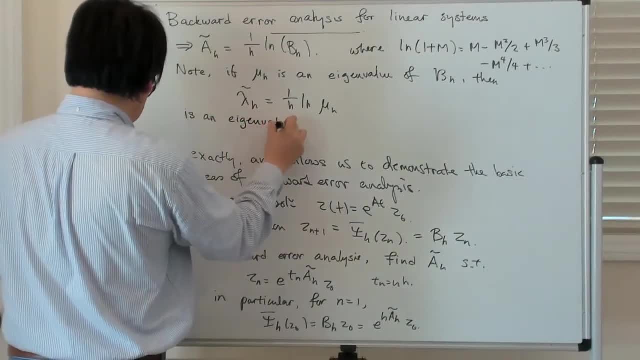 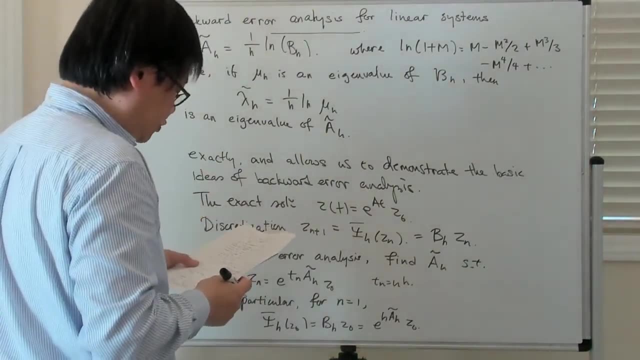 So we have, let's put a Timothy H to the 4 over mu, f over h a h tilde, And of course this is nothing more than the relationship between eigenvalues of a map and its associated linear operator. Okay, 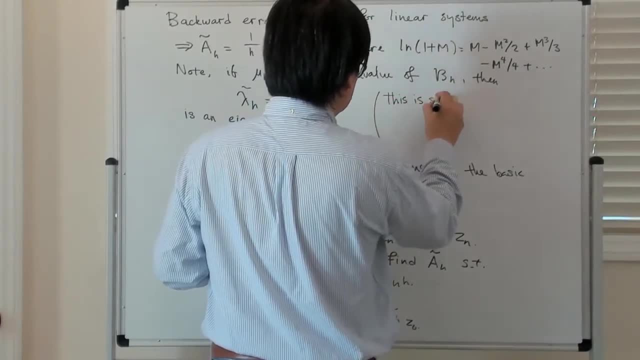 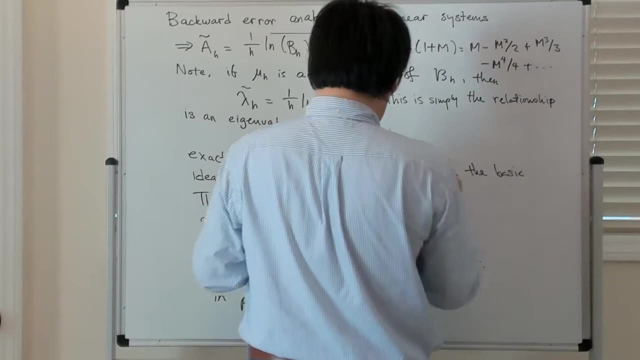 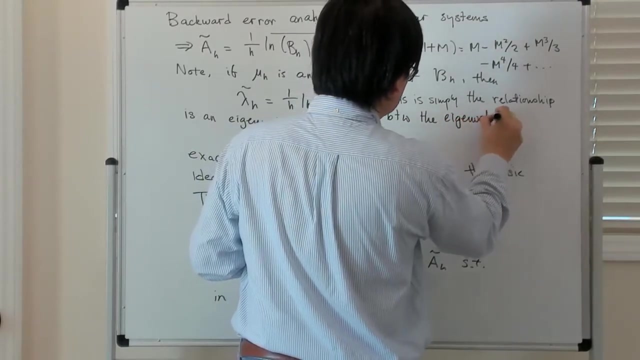 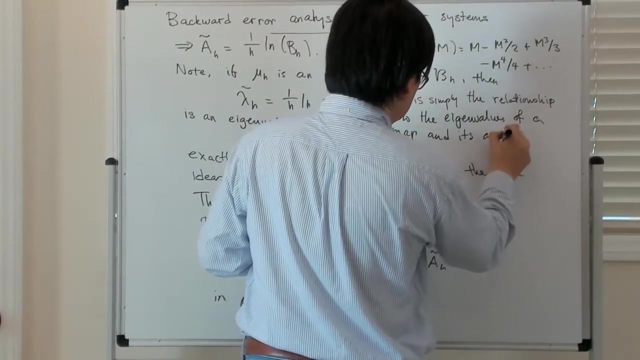 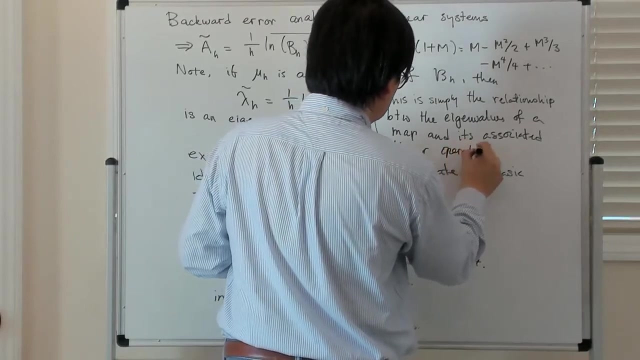 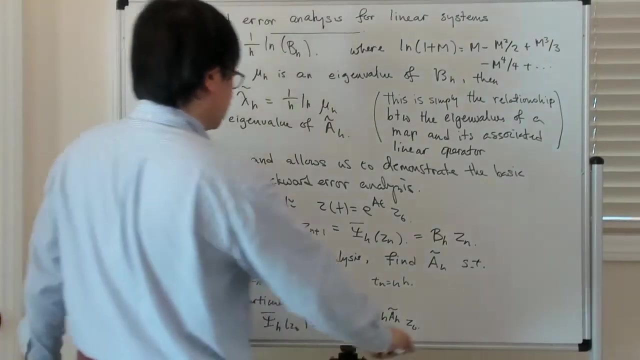 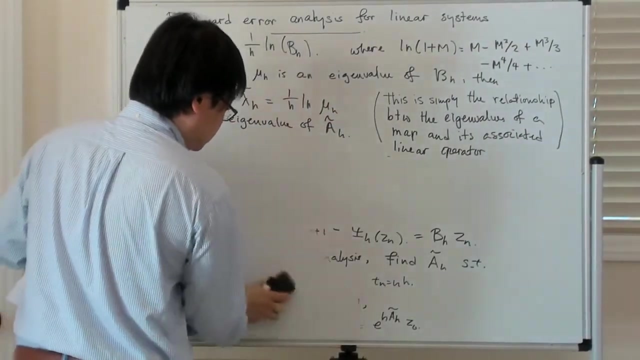 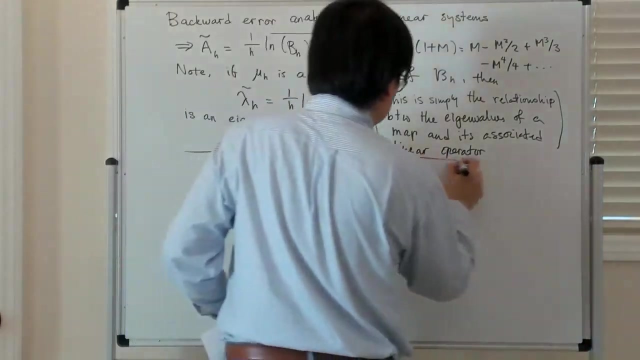 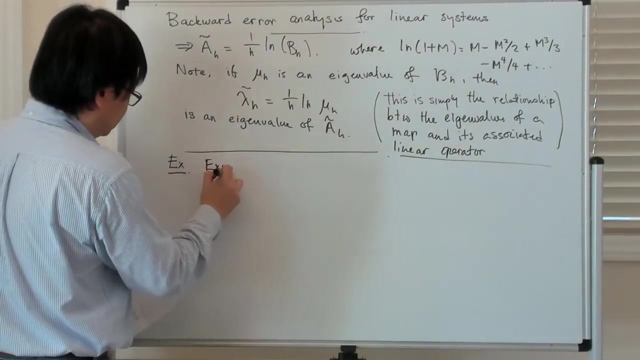 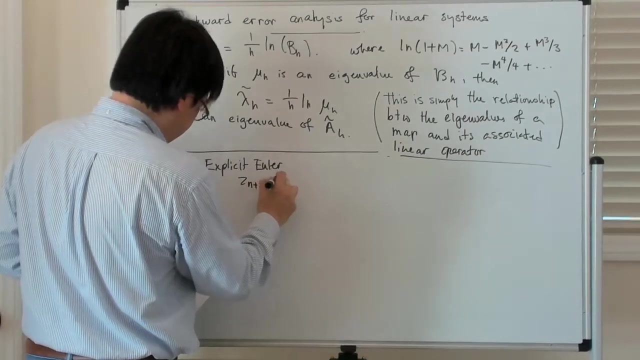 So this is simply the relationship Between the eigenvalues values of a map and its associated linear operator. So maybe it would be helpful to look at an example of this. Okay, so let's look at explicit Euler, right? So Zn plus 1 is equal to Zn plus Hacn. 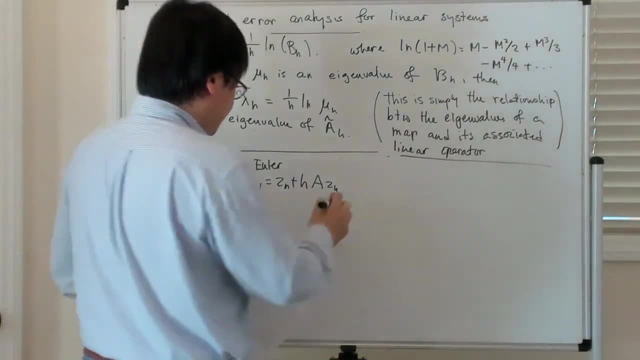 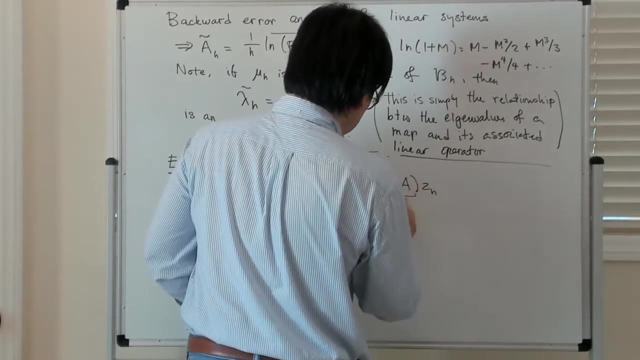 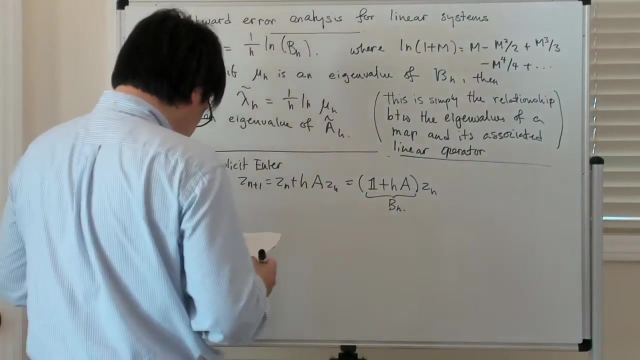 So you want to write this as a linear operator. This is a linear operator acting on Zn. This is just the identity plus Ah acting on Zn. So this is what I had called Bh, basically. Okay, so let's consider the harmonic oscillator. 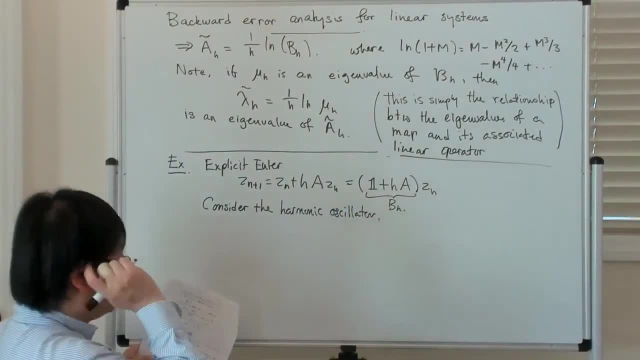 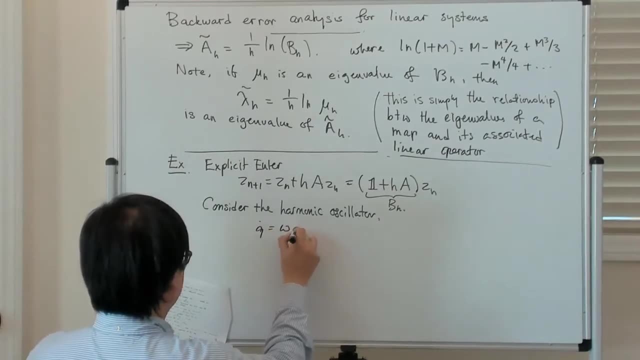 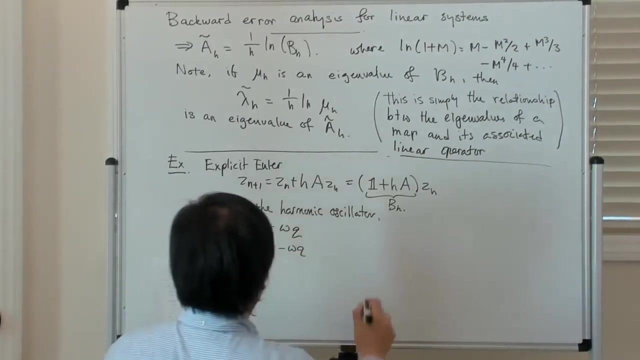 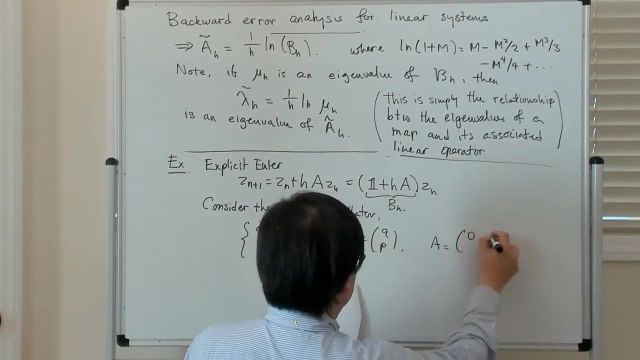 Okay, So I'm essentially looking at a specific choice of the A. Okay, so you have: Q dot is equal to omega Q and P dot is equal to minus omega Q. So Z is Q and P, and then A is 0, omega minus omega 0. 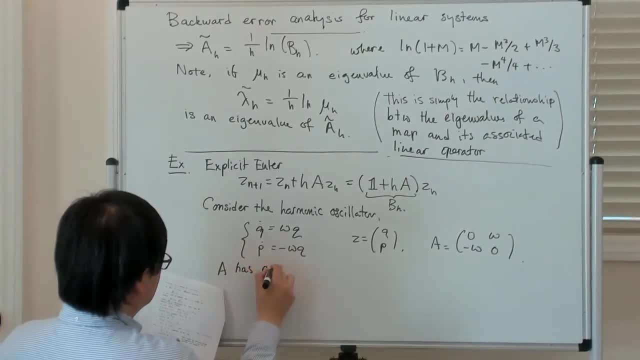 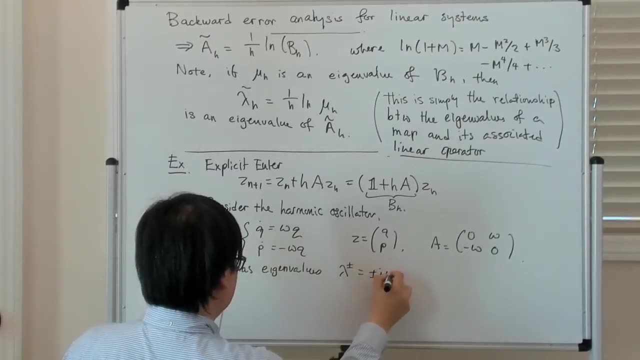 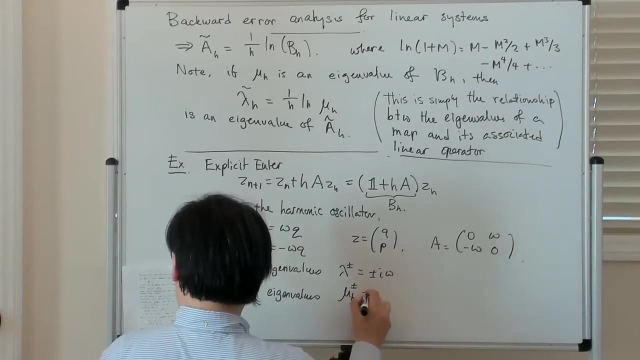 So you know that A has eigenvalues. Okay, Okay, Okay, Okay, Okay Okay. Lambda plus minus, which are just plus minus I omega. All right. And then Bh has eigenvalues. Let's call them mu, H plus minus, which are 1 plus minus I omega. well, I omega H. 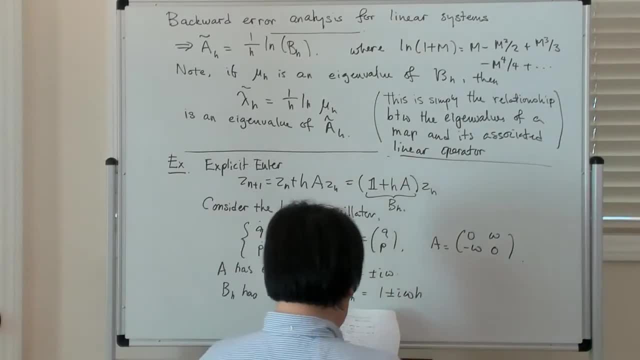 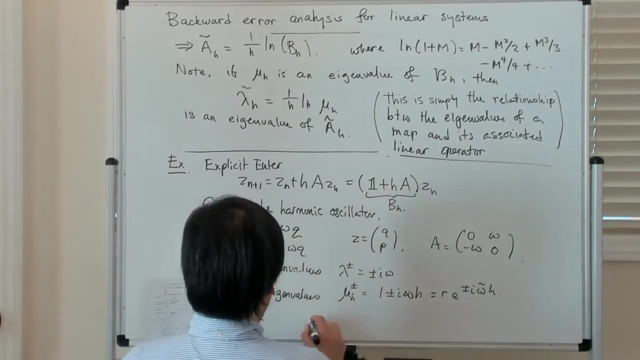 Okay, So so I can write this as Re to the plus minus I omega tilde H. okay, where, oops, R is equal to square root of 1 plus H omega squared, and then omega tilde right is equal to the R10 of omega squared. 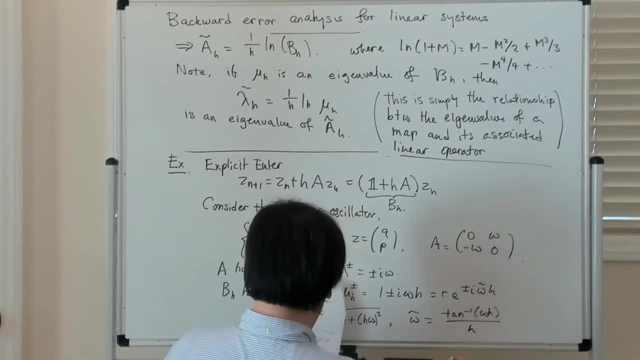 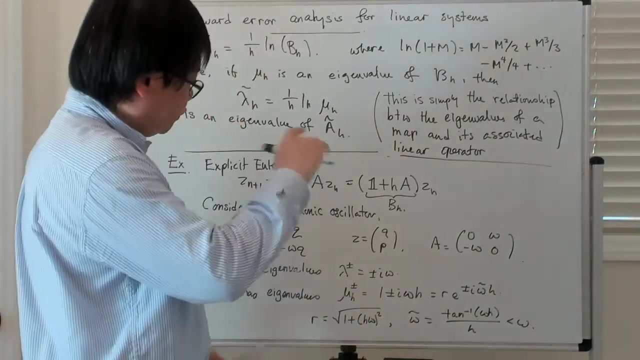 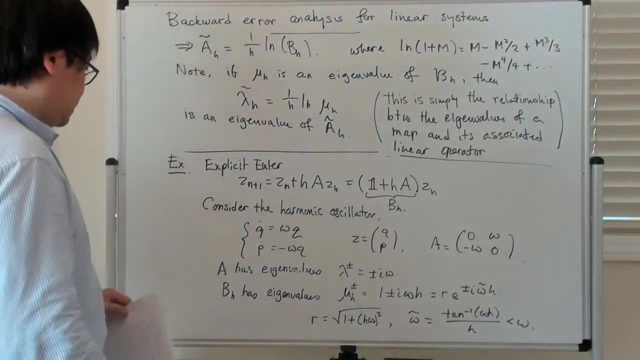 Okay. And then if you look at the series expansion for this, it's like you can conclude that this is less than omega Okay. So so what does that allow you to say? Right, So the radius is increasing, right And like with the harmonic oscillator, where it's like in phase space, it's like, you know, it's like the, the system doesn't, you know, it's like the orbit sort of doesn't grow. 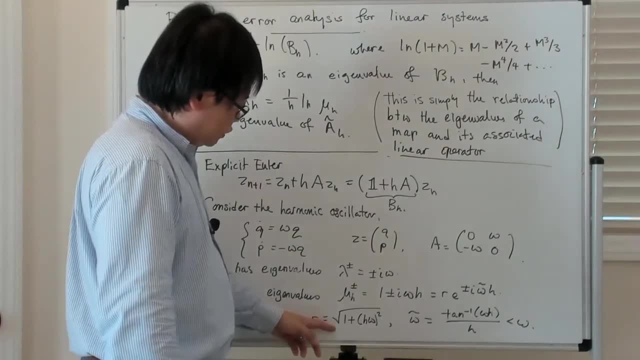 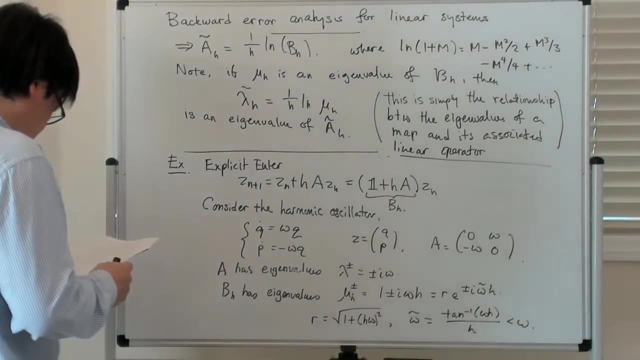 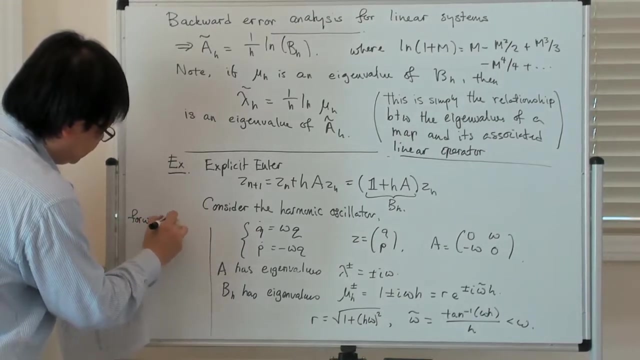 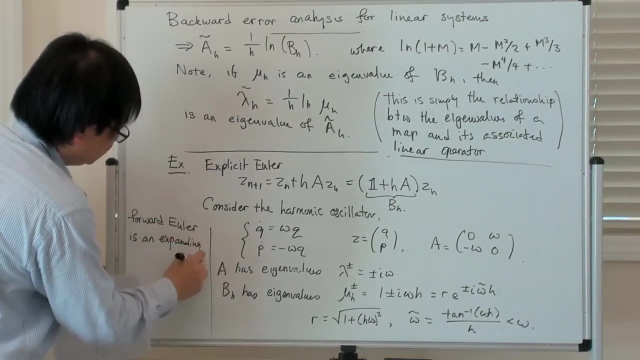 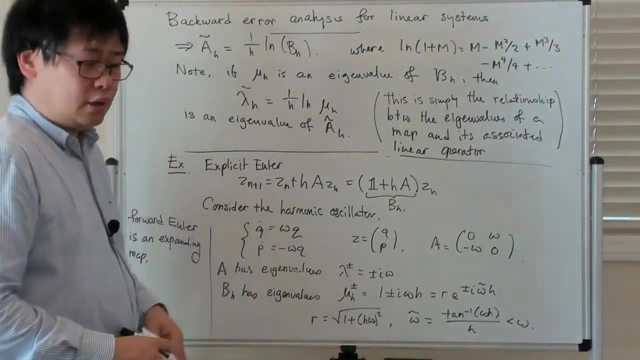 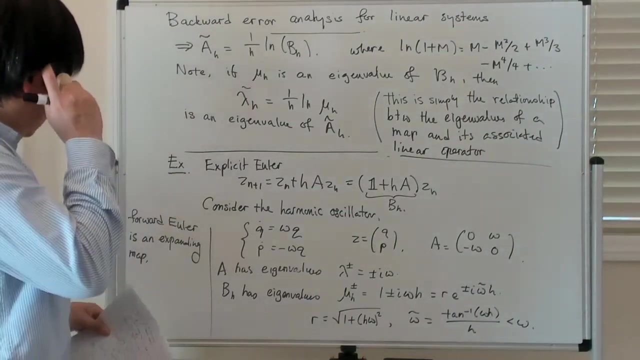 in the Ford Euler discretization. the radius of this thing is growing and then the frequency is slower. okay, so so basically, the conclusion is that Ford Euler is an expanding map, whereas the exact flow of the harmonic oscillator is not expanding right. its eigenvalues are purely imaginary, so it's neither growing or decaying. but with the 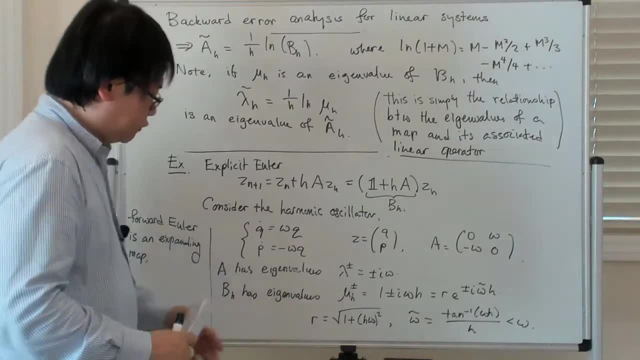 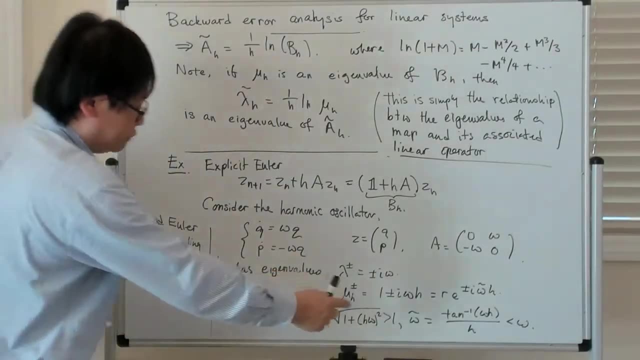 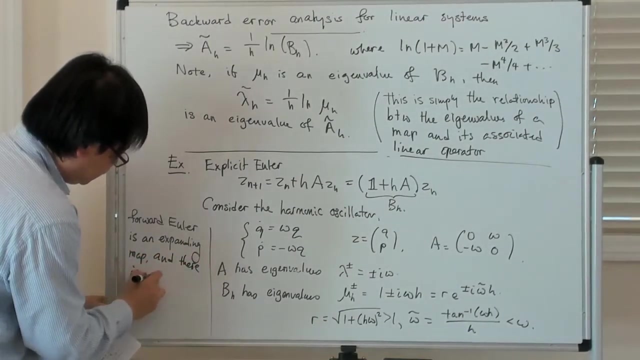 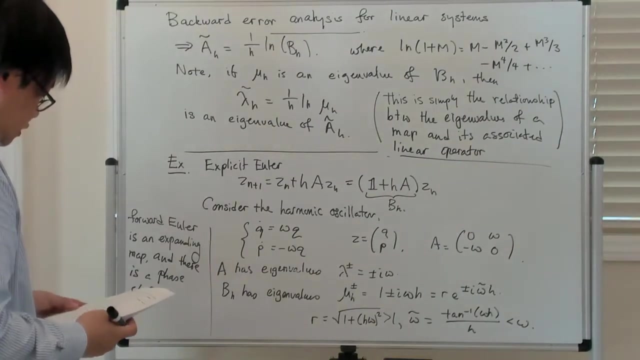 Ford Euler. it's like method. it has this sort of growth factor, so I should say that's greater than one right. it's greater than one right and there is a phase shift, because Omega tilde is not equal to Omega. okay, all right, okay, so let's just stop here. for now it's like, and then later. 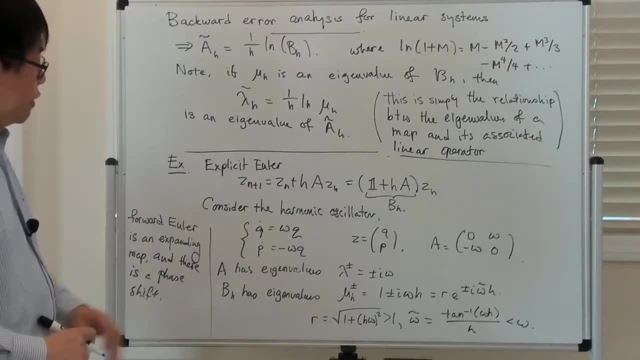 we'll look at a more general sort of from Cucuta method applied to the harmonic oscillator.